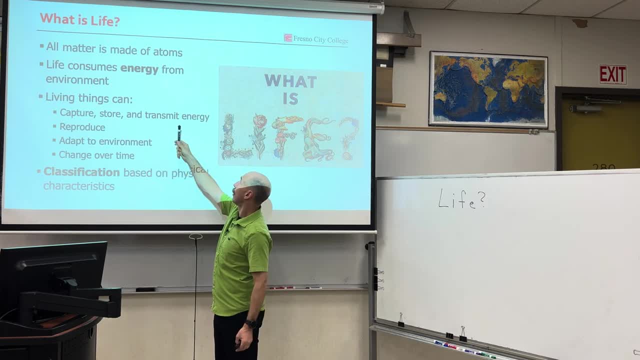 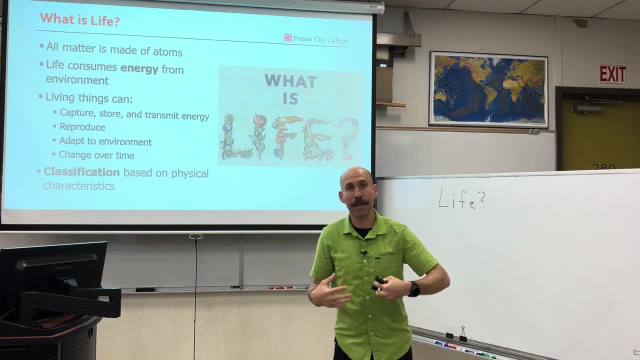 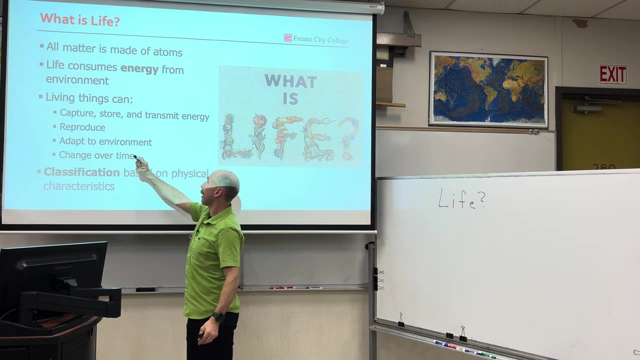 life is empty. Anything good- That's what a working definition says about life- is that we live in space. Now, מה life can be 삶? as if 25% had adapted to the teaching at Lu Long Fen. and one note is ancient facts: Life can change as long as 20,000ARS has, because that's what it meant to live. 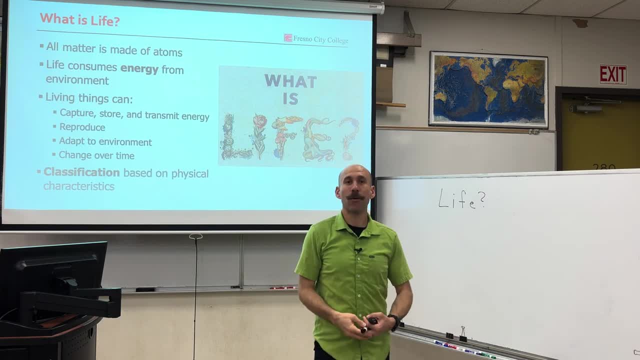 Life can be something. Life living things. Life can capture, store and transmit energy. plants capture energy from the sun. they store it, They transform it into usable energy sugars that are cri living things. life can capture, store and transmit energy. Plan and transmet engineering. plants capture energy from the sun. they store it, They transform it into usable energy sugars that are consumed by someone like you or me. like can't reproduce, But when life is adapted by life, like can change over time and we can class CVY11.我 Yesterday было. 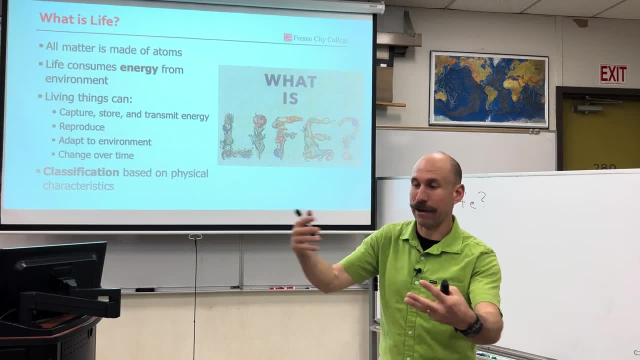 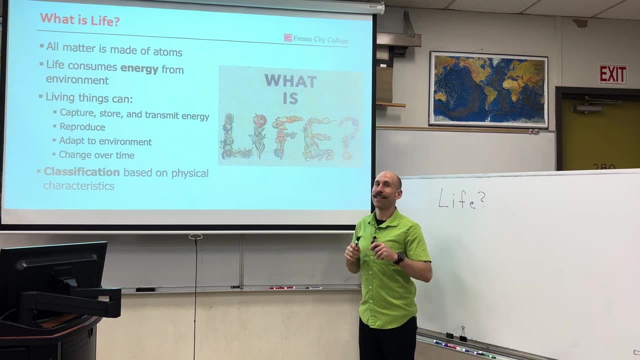 lirici我今天是生物生活的. I am a mammal animal, I have four limbs, so on and so forth. life, very scientific life is way more romantic and intentional. but for the purpose of marine life, what lives in the ocean? is the water alive? the water is not alive. the water holds life. let's 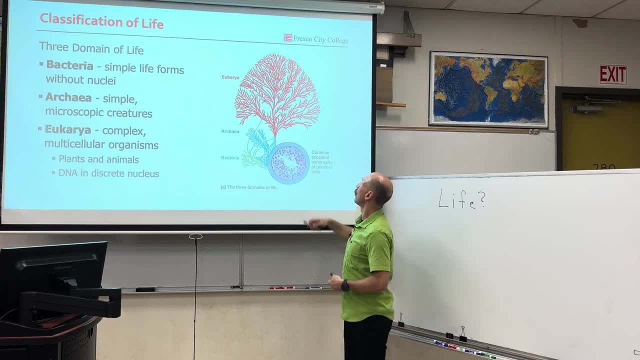 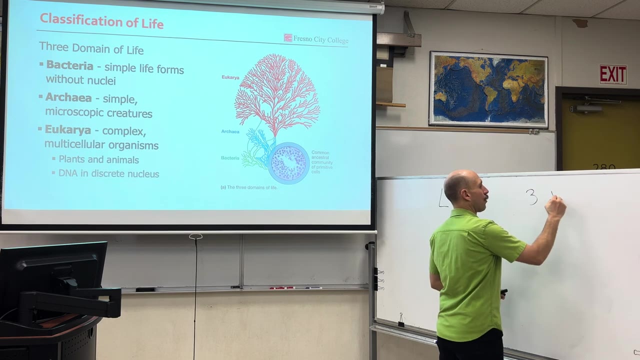 do a quick little overview three domains of life. we have eukarya, complex multicellular organisms. archaea, simple microscopic organisms. bacteria, simple life forms without a nucleus. so the three overarching domains of life. humans were in the eukarya domain. another way to look at this is we take all the life. 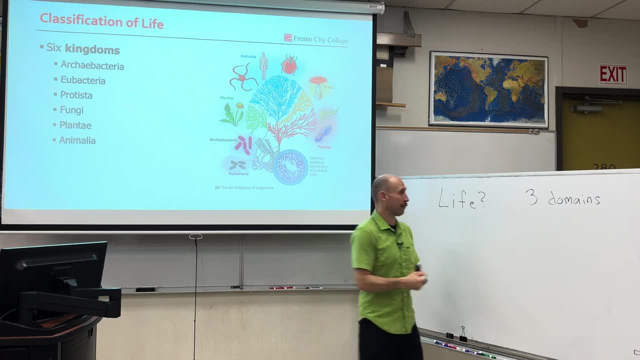 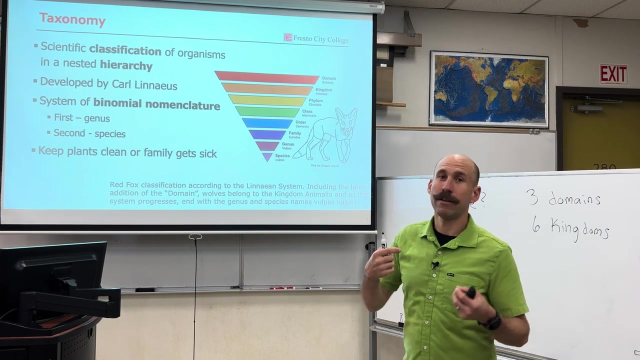 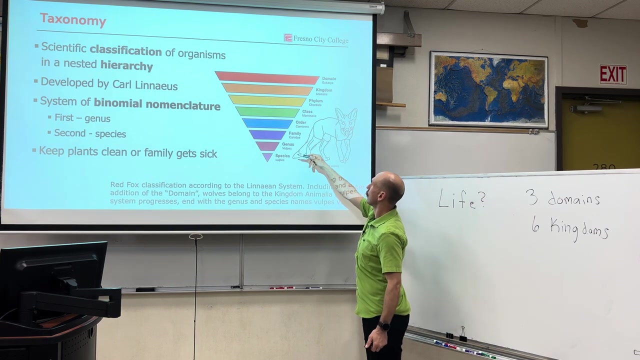 and we turn it into six kingdoms: protists, fungi, animals, plants, archaea, bacteria and you, bacteria. classification is hierarchical, based on physical characteristics: domain, Kingdom, phylum, class, order, family, genus, species. when we talk about different organisms, different species when we talk about different organisms. when we talk about different organisms. when we talk about different organisms. 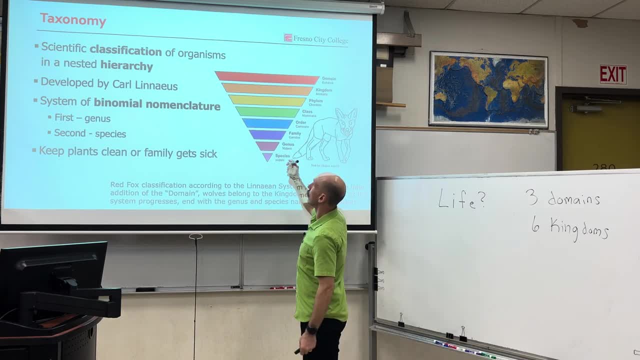 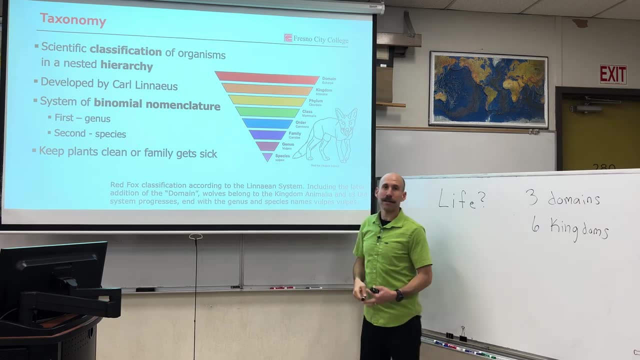 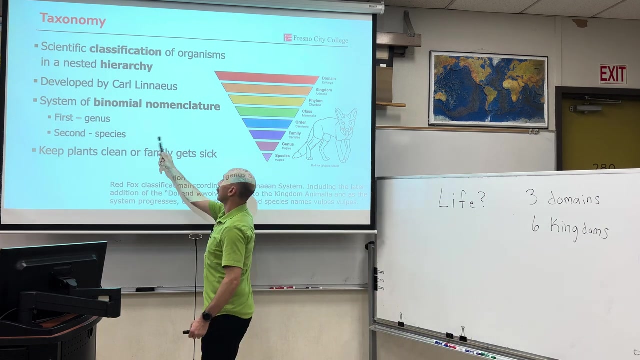 we can go back to the Linnaean binomial nomenclature. Carl Linnaeus is a individual who, basically, was the first person to catalog all the known species at one time and put a very specific way of identifying them that could be universally used. and we still use this system today. we go genus, species, humans. 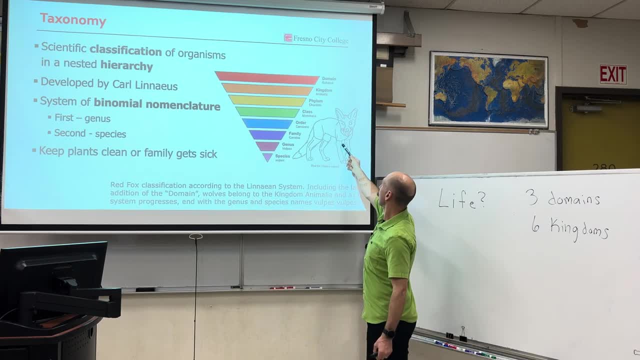 are Homo sapiens. in our example here we have a genus called Homo sapiens and we we have a genus called Homo sapiens. in our example here we have a genus called red fox is vulpus. vulpus, and you can remember this: keep plants clean or family. 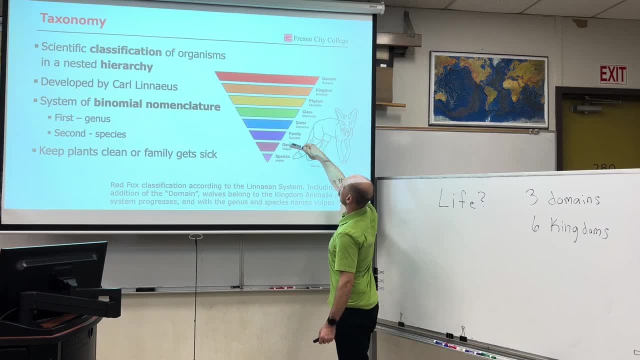 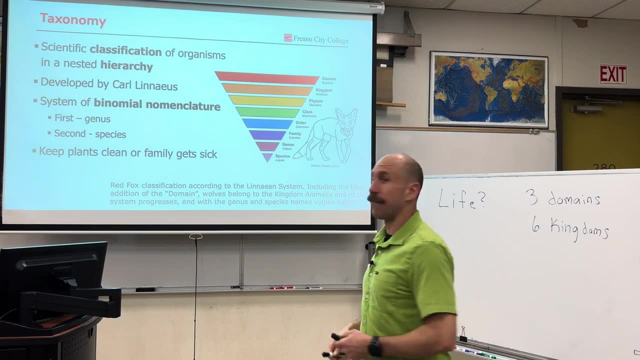 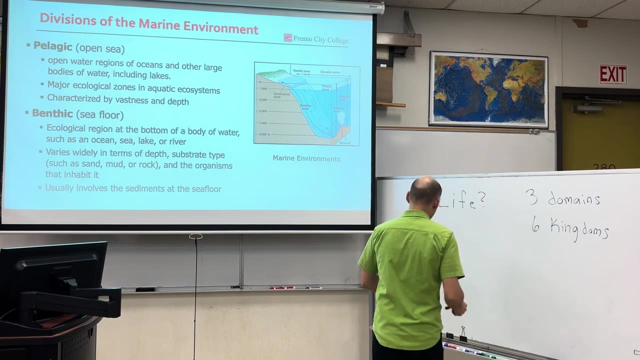 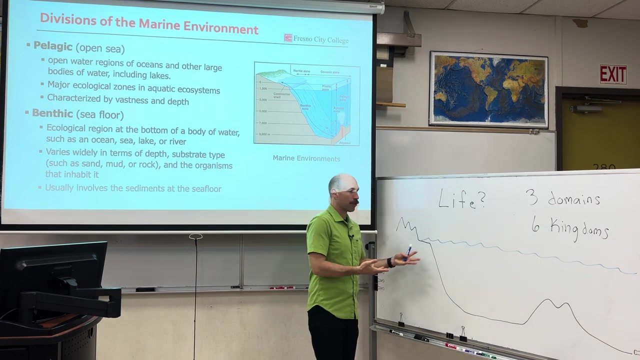 get sick. that is kingdom, phylum class order, family, genus, species. keep plants clean or family gets sick. cool, great. so we've defined life, we've figured out how we classify life. now let's take this to the marine environment. this is my favorite cartoon image drawing ever. Do you remember what this is? This is the. 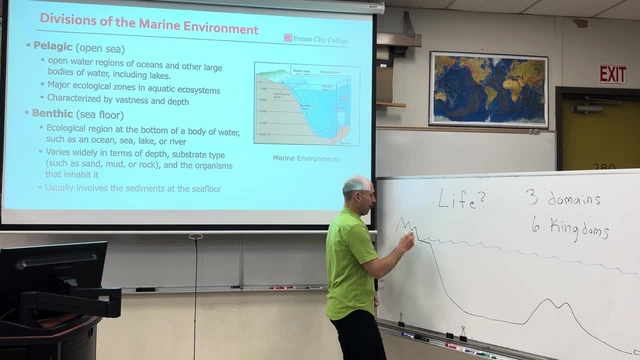 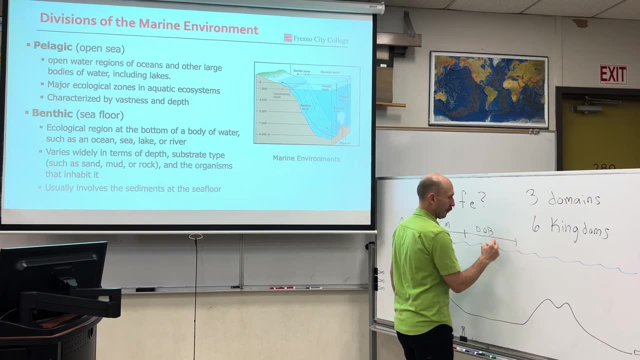 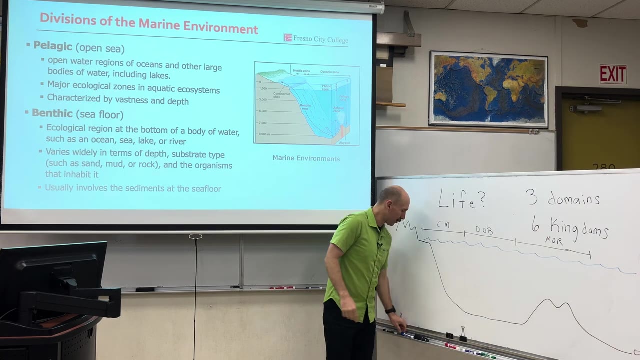 structure of the ocean, where we have the continental margin, the deep ocean basin and the mid-ocean ridge system. Now we are going to break this out into two divisions: The ocean floor all the way along, the entire ocean floor. do-do-do-do-do-do-do-do-do. 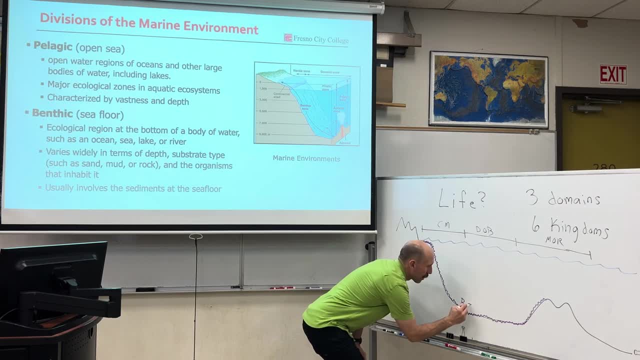 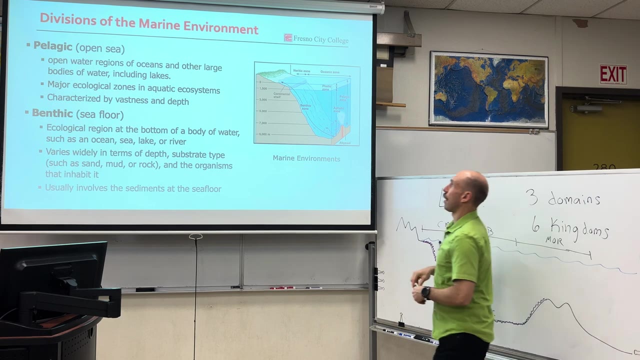 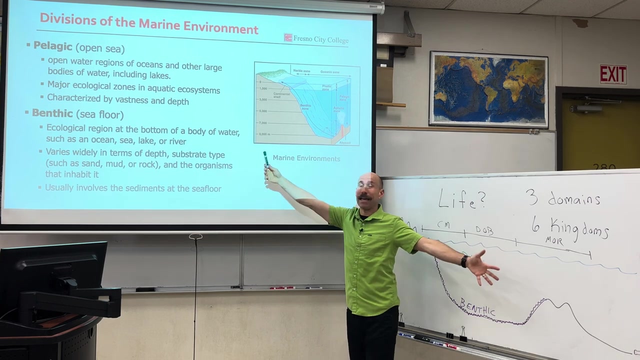 so on and so forth. We'll call this the benthic environment And the rest of the ocean the open ocean. we'll call the pelagic environment, Pelagic, open water region, major ecological zones by depth, characterized by how big it is, Benthic. 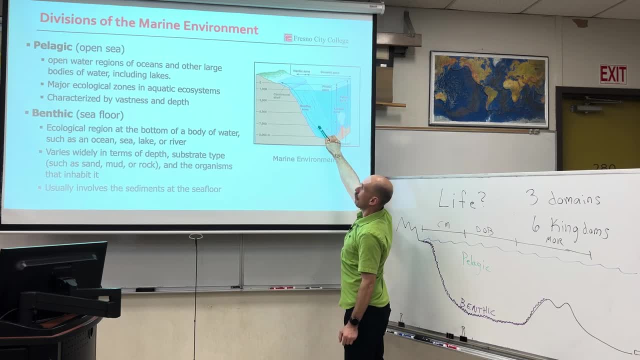 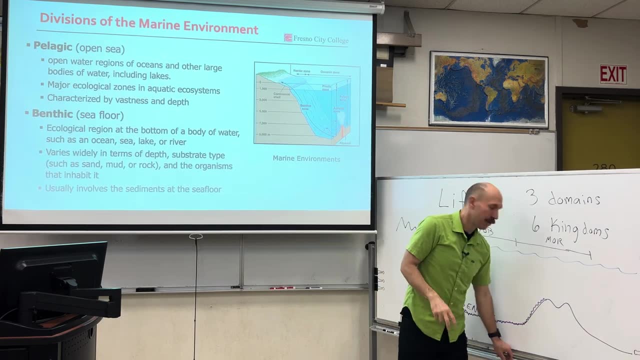 it's at the region. ecological region at the bottom of the ocean varies widely in depth, substrate type. Usually the bottom of the ocean is very big, very shallow, very deep. involves either rocky bottoms or sediment cover bottoms which will give 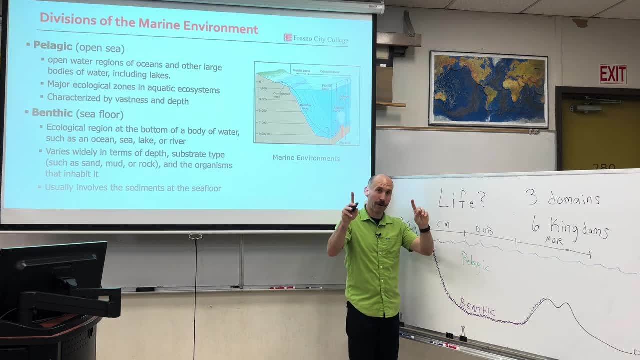 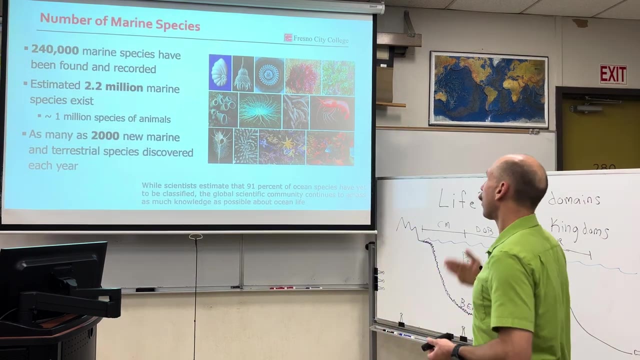 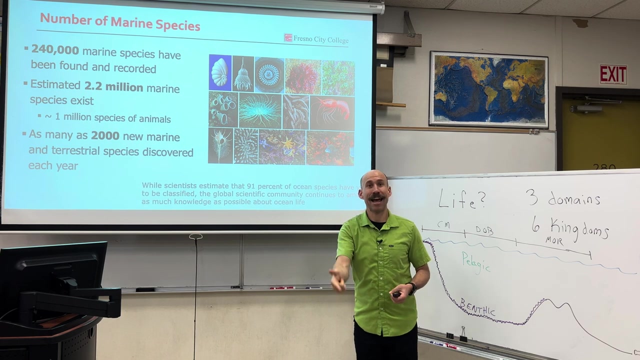 us different types of species, but this is the important part. when we think about marine life, we are looking at the pelagic environment and the benthic environments. so how many species are there? excuse me, currently 240,000 marine species have been identified and catalogued, but the estimates for how? 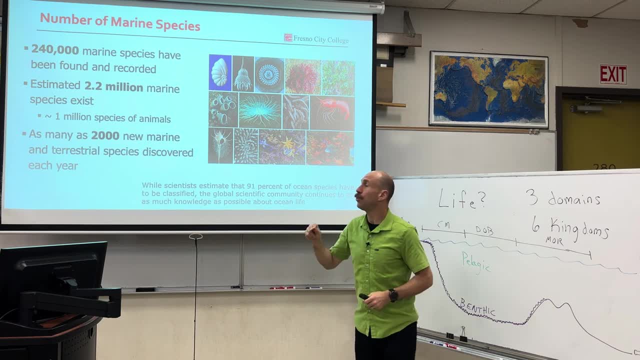 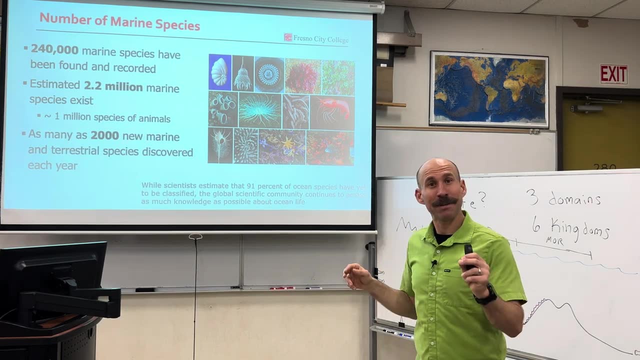 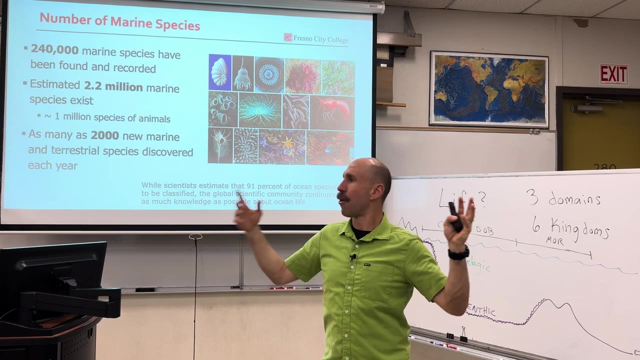 many species are in the ocean range at about 2.2 million, so we have only found a fraction of what is believed to be existing in the ocean. that's awesome: the ocean, last great frontier. exploring the ocean bottom, working in marine biology, finding out what's there. every year, 2,000 new marine and terrestrial species. 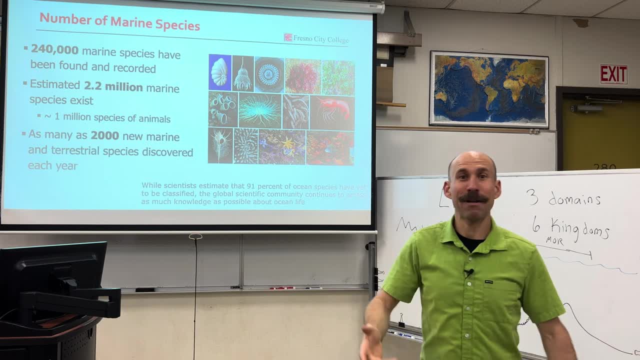 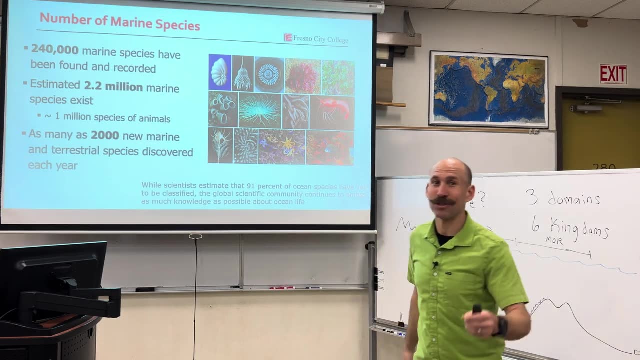 are discovered- and the ocean is the world's largest marine and terrestrial species are discovered. this could be you. you could have a marine animal named after you that you discover 35,000 feet below the surface of the ocean, in the deepest place that we know of the Mariana Trench. it's out there, it's. 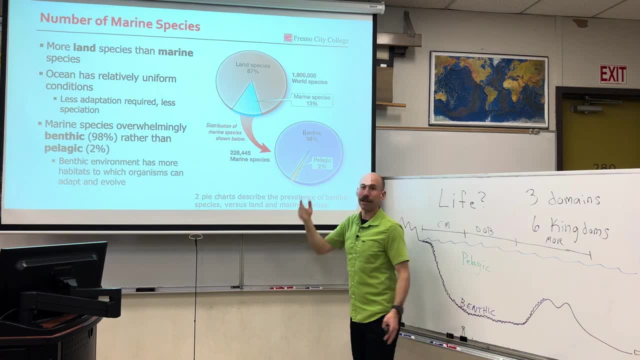 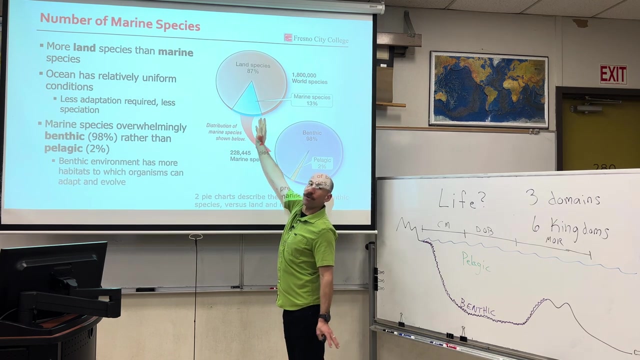 available. so here comes our benthic and pelagic. overwhelmingly, marine life exists in the benthic environment. there's more habitats for species to adapt and evolve, to diversify. so let's look at this one total biodiversity: 87 percent of the species live on land, about 13 percent. 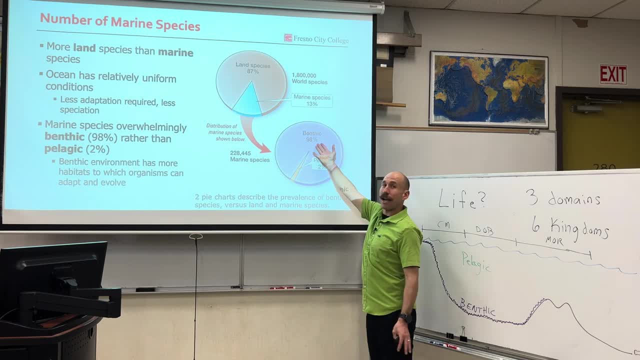 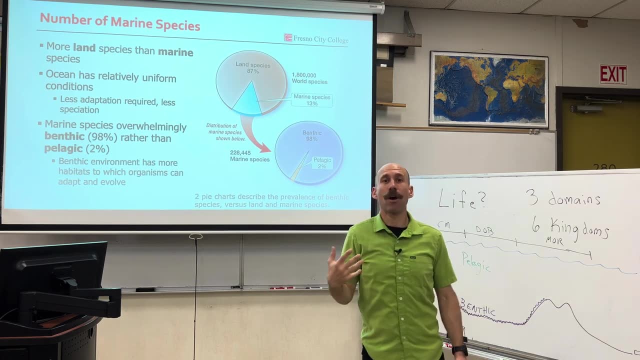 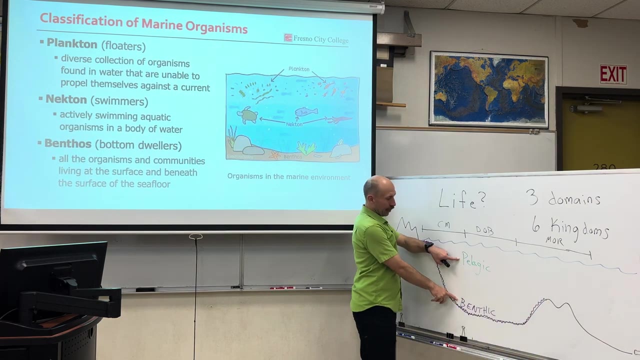 live in the ocean. of that, 13 percent. 98 percent live on the ocean floor, in the benthic environment, and two percent live in the open ocean, in the pelagic environment. here's our divisions: benthic and pelagic. now let's classify marine life and we 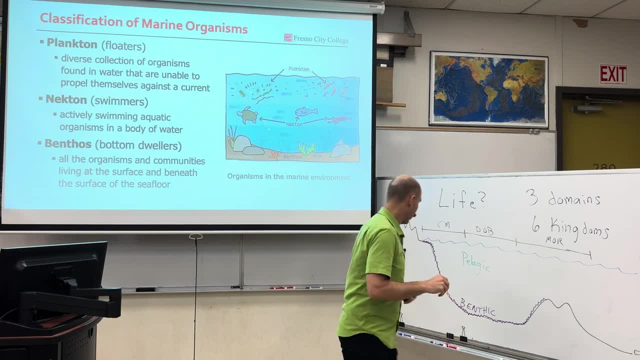 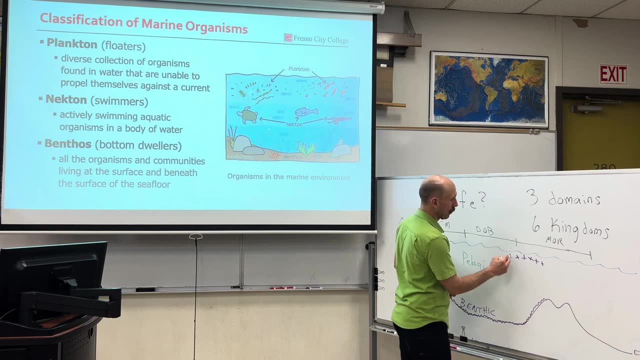 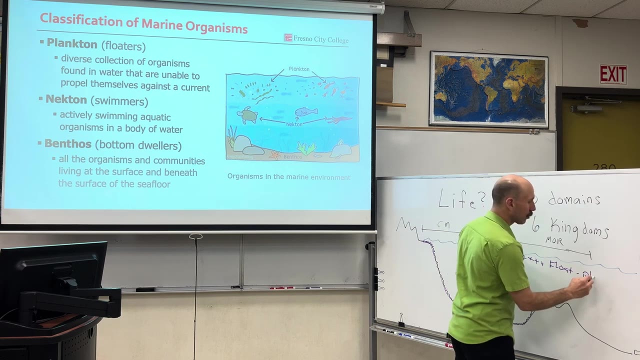 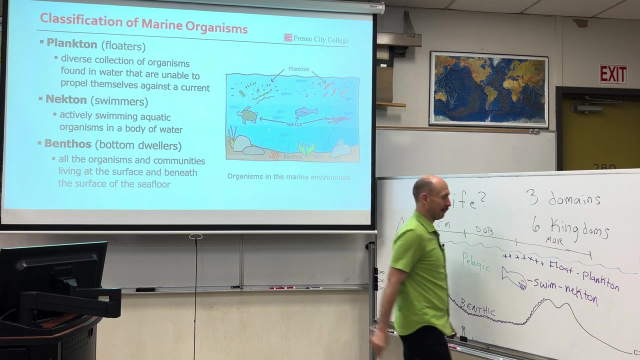 are going to put three main classifications on them. we have organisms in the ocean that float, and floaters are called plankton. there are organisms that swim, and we call swimmers nectin. and then we have organisms that live on the bottom of the ocean, in the benthic environment, and we call them benthos. 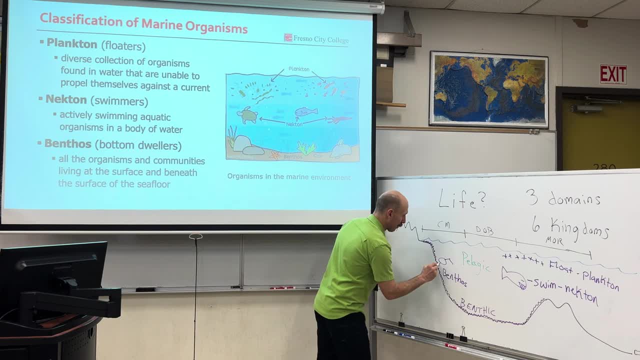 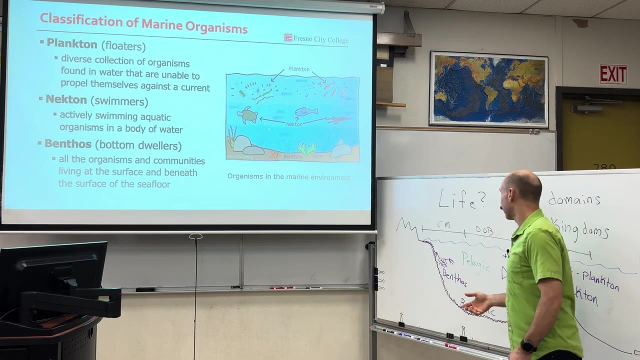 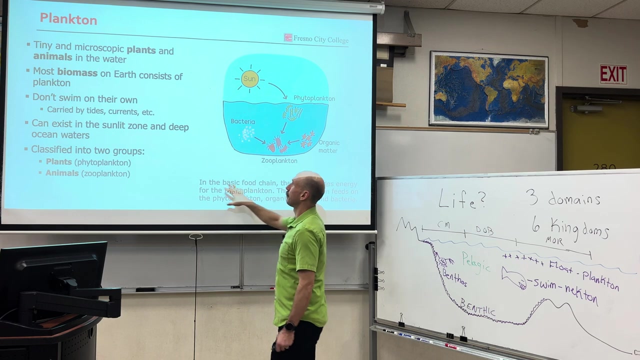 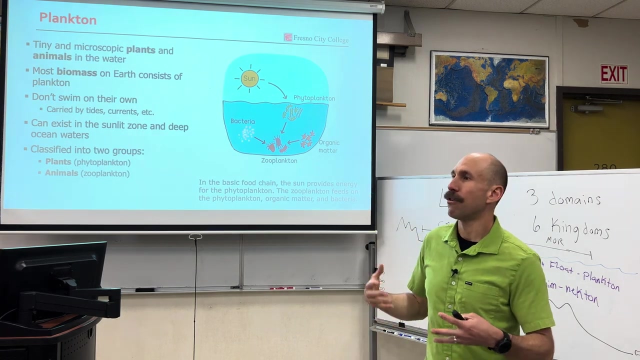 should I do something like this? that's a crab. that's a horrible crab anyways. so three types of marine organisms: floaters, Swimmers and Bodom dwellers. now Let's talk about plankton. plankton have Marine adaptations in size and body shape in order to float. 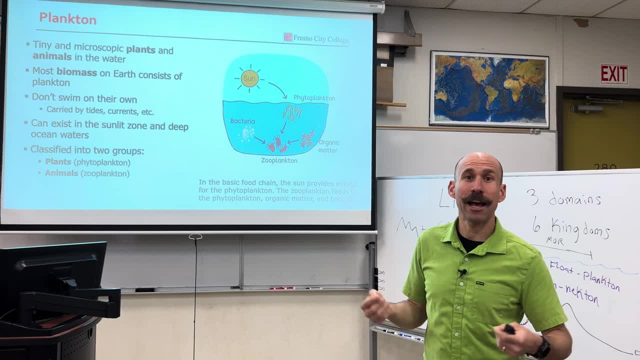 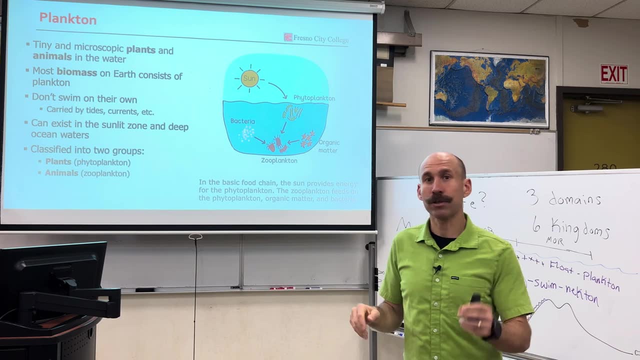 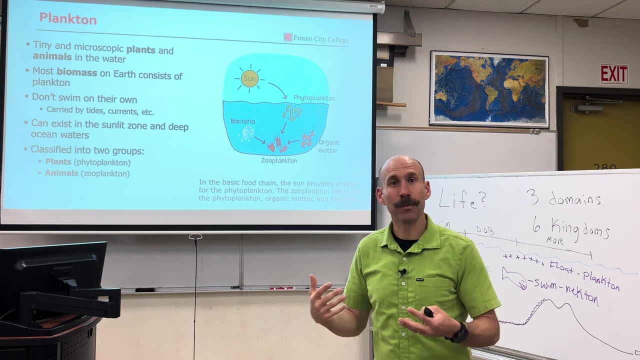 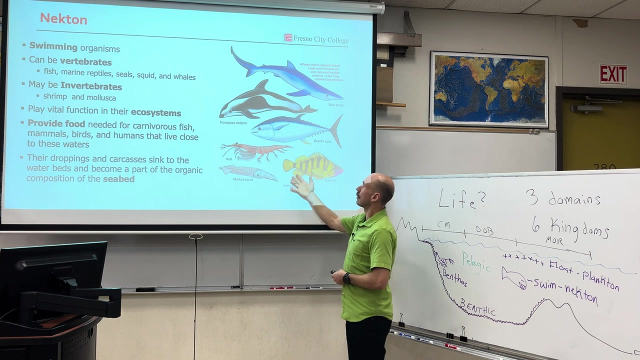 they drift with the currents of the ocean and the tides. phytoplankton are marine photosynthesizers that are eaten by primary consumers, zooplankton. these form the base. the base and the first level of the food web that, for that, feeds marine organisms. nektin. this is going to be all of our swimming. 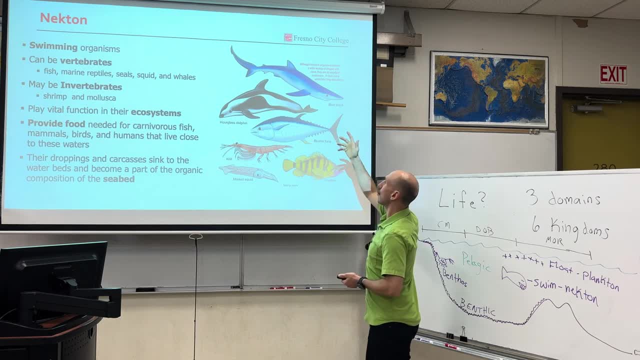 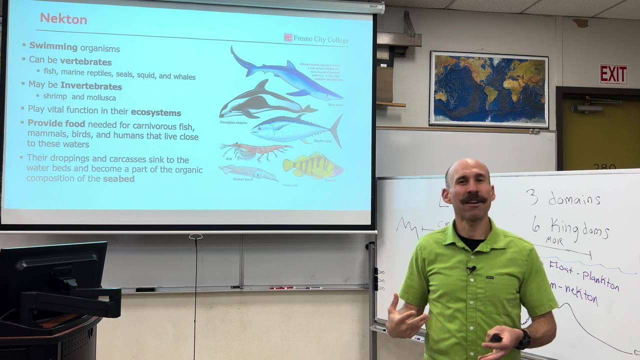 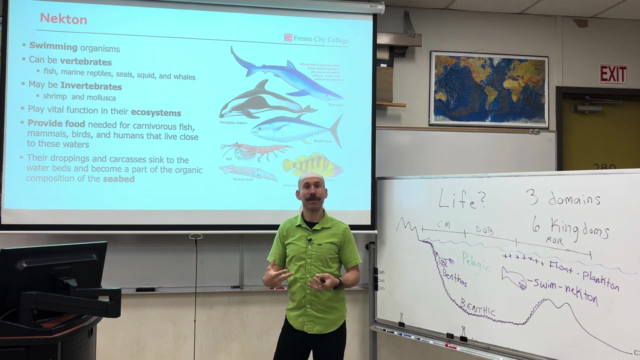 organisms. we've got fish, we've got whales, we've got invertebrates, meaning reptiles, seals, squids, all of the above. this is an important component of the food web, because the nektin are going to eat a lot of the floaters. their droppings and carcasses will sink to the bottom and become marine sediments, which 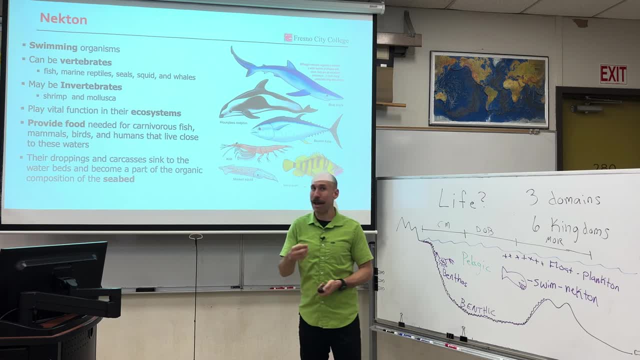 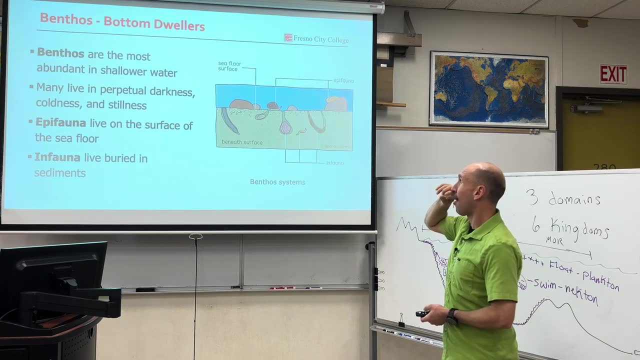 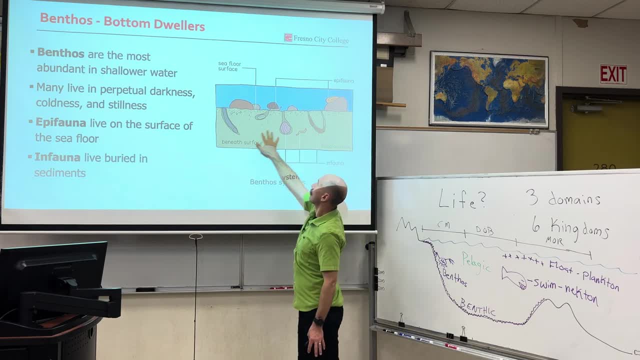 environments. we have two types of environments. we have two types of benthos benthic organisms that burrow benthos benthic organisms that burrow benthos benthic organisms that burrow down into sediment. we call this in fauna- down into sediment. we call this in fauna. 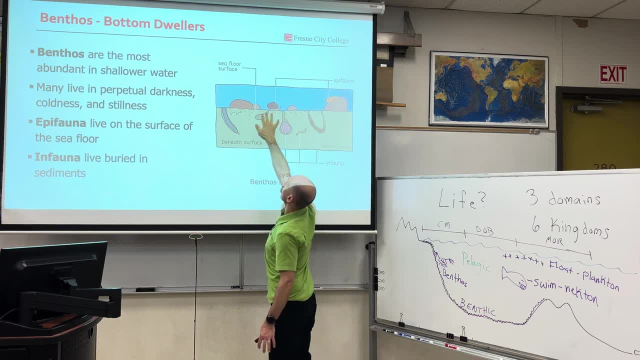 down into sediment. we call this in fauna and benthic organisms that live on top of, and benthic organisms that live on top of, and benthic organisms that live on top of the seafloor surface, the seafloor surface, the seafloor surface. we call them epiphauna. so let's see so. 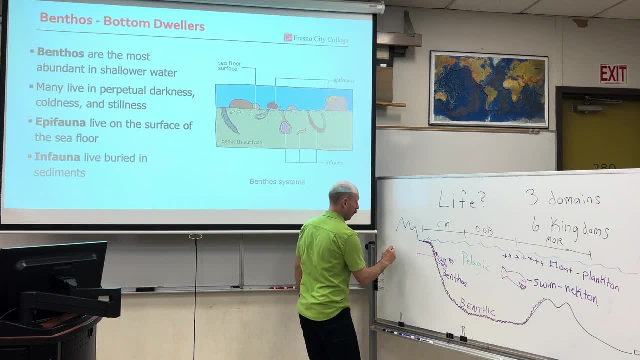 we call them epiphauna, so let's see. so we call them epiphauna, so let's see. so this little crab, this would be epiphauna. this little crab, this would be epiphauna. this little crab, this would be epiphauna. and in fauna, I apologize about the red. 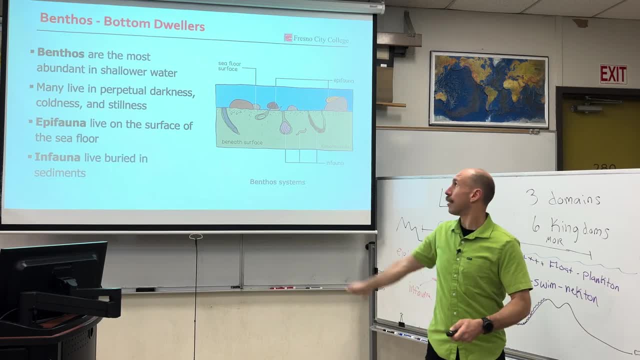 and in fauna, I apologize about the red and in fauna, I apologize about the red pen. hopefully you can see this. it looks pen. hopefully you can see this. it looks pen. hopefully you can see this. it looks like it's not coming out very well. let's like it's not coming out very well. let's. 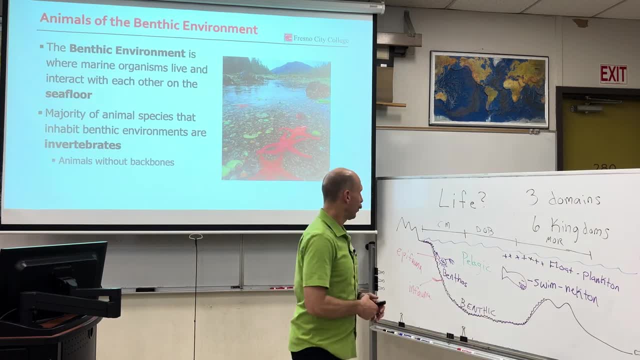 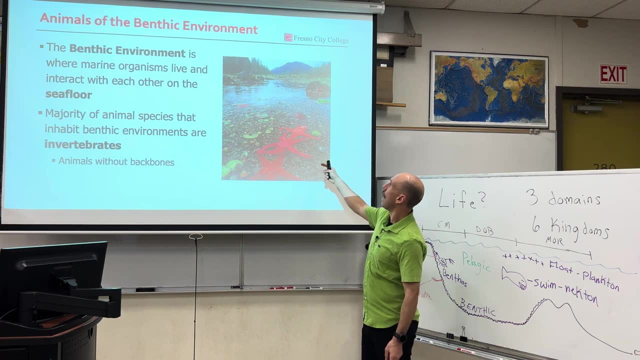 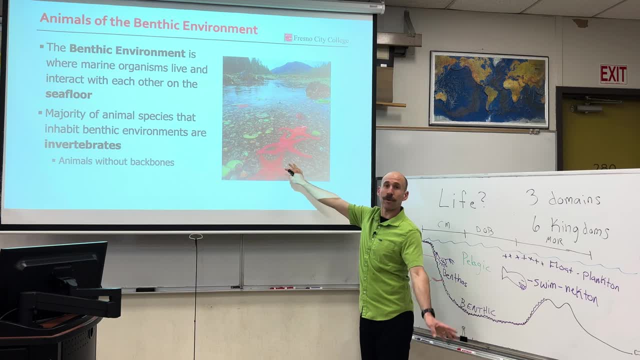 going to have many organisms living and going to have many organisms living and interacting with each other on the interacting with each other, on the interacting with each other on the seafloor. for the most part, this is where seafloor for the most part, this is where 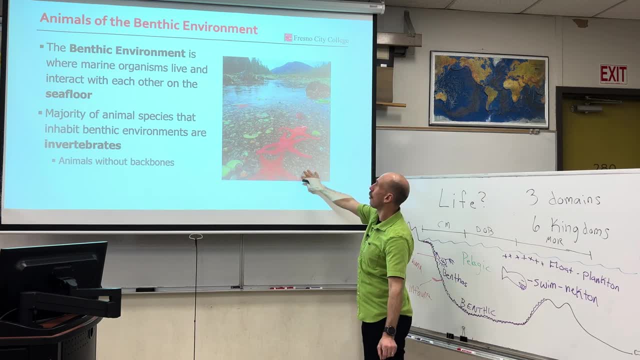 seafloor for the most part. this is where our invertebrates live animals. without our invertebrates live animals without our invertebrates live animals without backbones, creating a suite of various backbones, creating a suite of various backbones, creating a suite of various communities based on how deep they are. 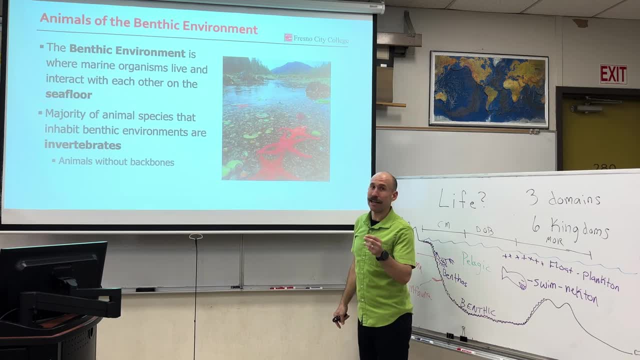 communities based on how deep they are. communities based on how deep they are in the ocean. really associated with in the ocean, really associated with in the ocean. really associated with high tide, low tide, sub tide, super tide, high tide, low tide, sub tide, super tide, high tide, low tide, sub tide, super tide, and then sediment or rocky covered. 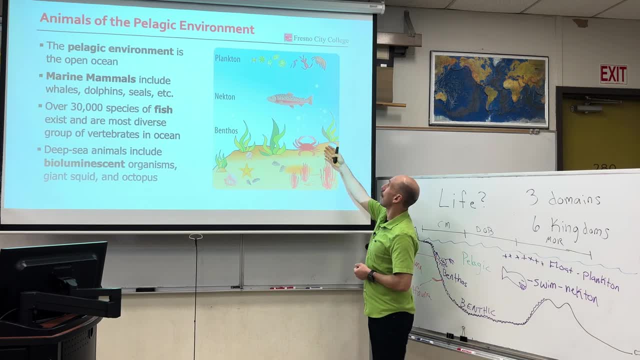 and then sediment or rocky covered and then sediment or rocky covered. shores, the pelagic environment, plankton shores, the pelagic environment, plankton shores, the pelagic environment, plankton and nectin- so big groups here are going. and nectin, so big groups here are going. 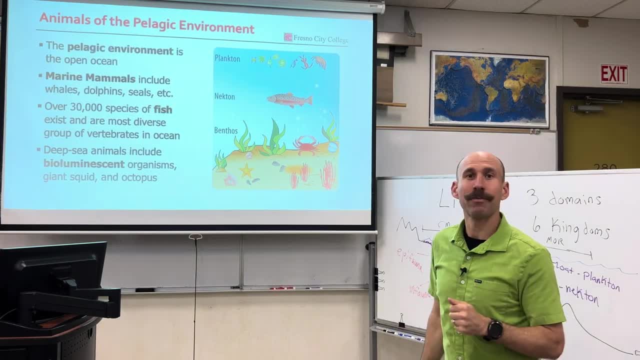 and nectin. so big groups here are going to be our phytoplankton, our zooplankton, to be our phytoplankton, our zooplankton, to be our phytoplankton, our zooplankton. and marine mammals, excuse me, marine. 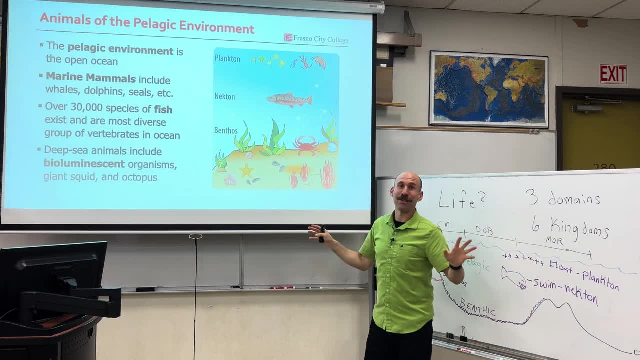 and marine mammals, excuse me, marine and marine mammals, excuse me. marine mammals and fish. lots of different types. mammals and fish. lots of different types. mammals and fish. lots of different types of fish in the ocean fish are awesome. of fish in the ocean fish are awesome. of fish in the ocean fish are awesome and extremely diverse. most diverse group. and extremely diverse, most diverse group and extremely diverse, most diverse group of vertebrates in the ocean. we go a of vertebrates in the ocean. we go a of vertebrates in the ocean. we go a little bit deeper in the ocean, we have. little bit deeper in the ocean, we have. 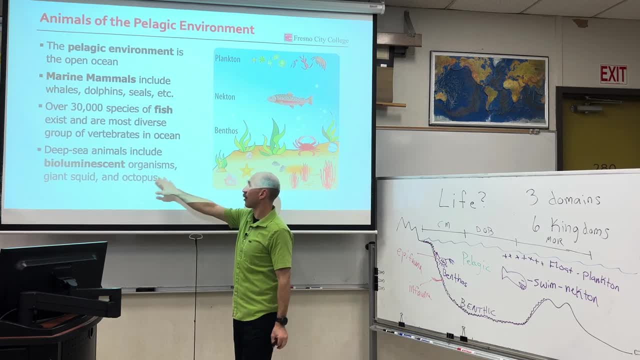 little bit deeper in the ocean. we have organisms that glow, bioluminescent organisms that glow, bioluminescent organisms that glow, bioluminescent organisms. we've got giant squid octopus organisms. we've got giant squid octopus organisms. we've got giant squid octopus- all kinds of cool animals, and we will. 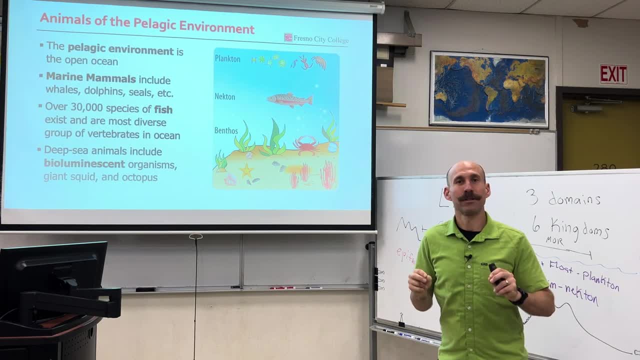 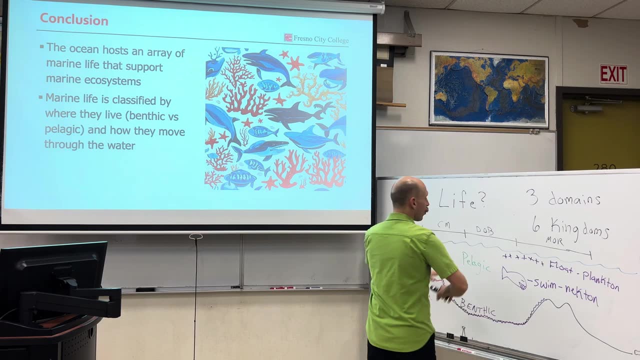 all kinds of cool animals, and we will all kinds of cool animals and we will have entire modules, subsequent lectures, have entire modules, subsequent lectures, have entire modules, subsequent lectures. from this point on where we discuss both. from this point on, where we discuss both. from this point on, where we discuss both marine life and marine life. life is made.